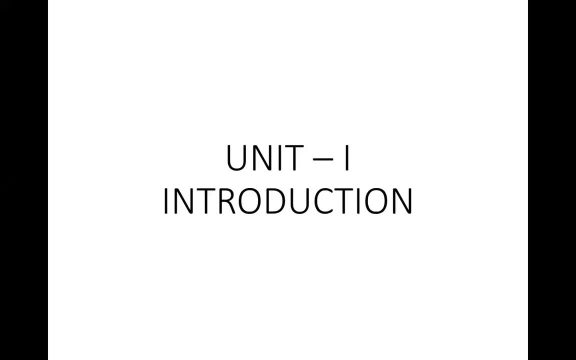 Thank you, Hello everyone. We will start with the unit number one. In previous session we saw the introduction of the subject, the importance of the subject about the result and everything. overview of the subject. Now, from today, we will see, or we will start the unit number one. The unit number one: the name itself is suggesting that this unit is introducing us about the human-computer interaction. 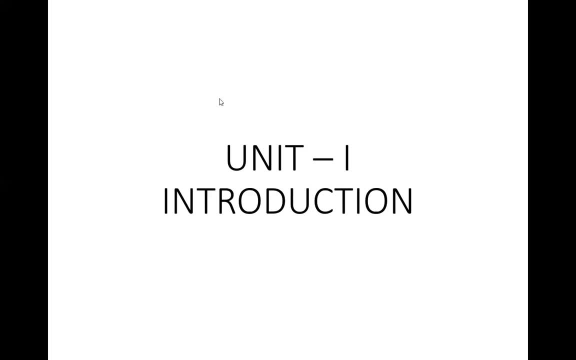 So let's see what exactly the HCI is. HCI- Human-Computer Interaction- The full form of the subject is HCI, that is, Human-Computer Interaction. So the name itself suggests that this is the interaction between the human being and the computer. Now, as our field is IT or computers, so the term computer is there. 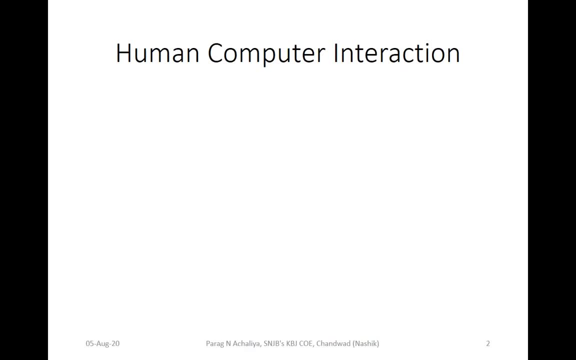 Otherwise we may call it as human-system interaction. So the system can be anything, The system can be the machine. But now we are specific, We are strict to our branch. So the HCI stands for Human-Computer Interaction. It is the interaction between the human and the machine. The machine can be your robot, It can be your computer system, It can be your vehicle, It can be your electronic device. 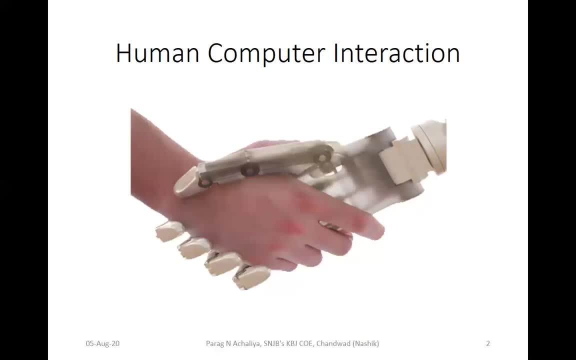 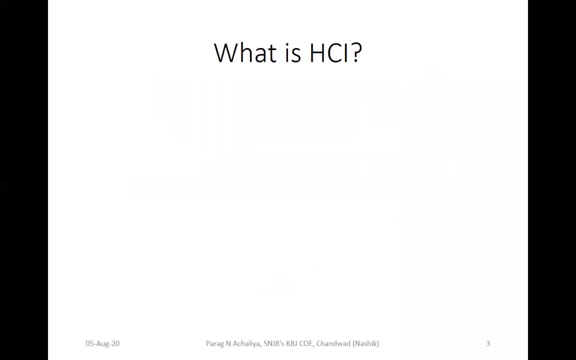 It can be your mobile, It can be your any object, anything, Anything comes into your system. So that is your HCI. So what exactly the HCI is? the term HCI has only been widespread since 1980.. First time this term was used as a Picture Maker in the 1980s. 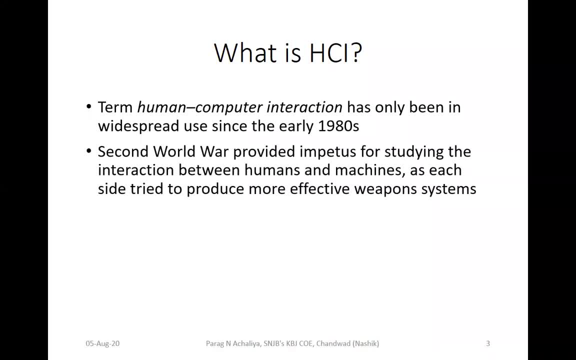 The Second World War provided impetus for studying interaction between humans and machines. as each side try to produce more effective weapons system, hci, both the sides have started using various types of weapons, huge amount of weapons, for the war purpose. so the human started using the weapons. for what? 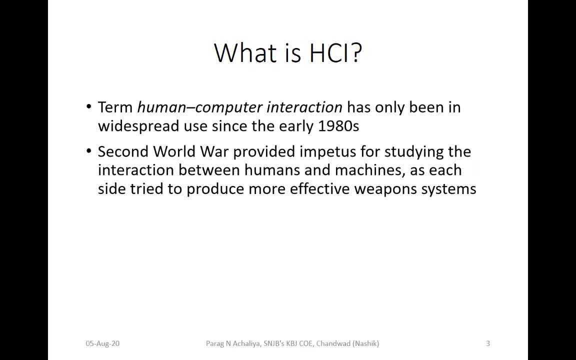 war. so there the human and machine are started interacting with each other. from second world war, or we can say since 1980, this term comes into the picture. this led to wave of interest in area among researchers where the researchers start doing their research in human and computer interaction. 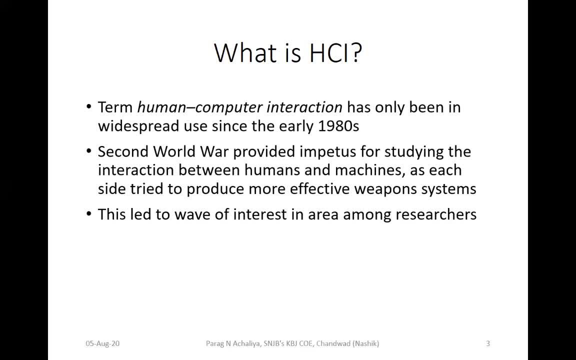 so many people completed their phds or research work in human computer interaction, how the human can interact with the system, how the human can interact with the computer. this is one of the interesting area where many people have achieved their phd. they became the phd scholar and now they are at very 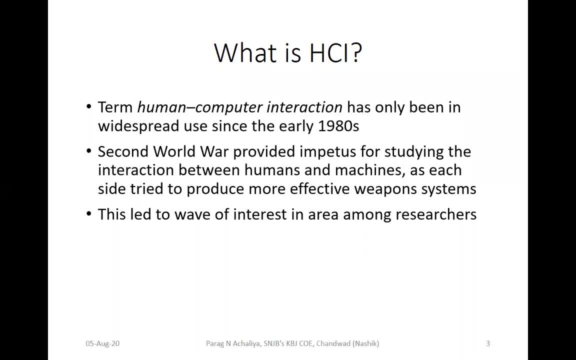 good position in research or as a researcher as computer use become more widespread. researcher studying interaction between people in the upper land, computer with physical, psychological and theoretical aspect of this process, as we discussed nowadays. you observe all the people living in institute in this 25 years more doctorsto end on and in all these volunteers. 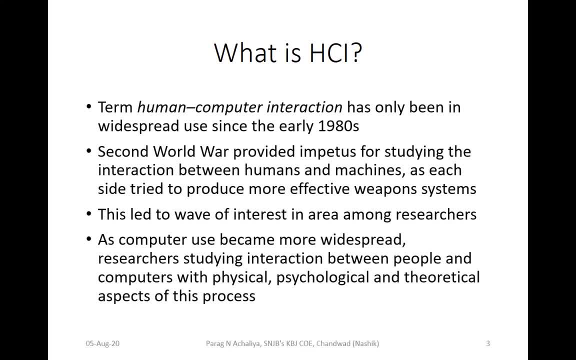 more oftenхay no more advanced. more often. andgardar: 95 or 100 percent of you people are attending this lecture. through what mobile device? i am the only person who is delivering the lecture from my pc, but you are attending your lecture from the mobile. 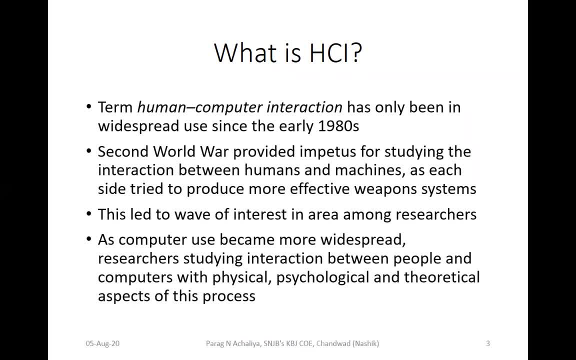 so that is why the computer is becoming what very famous or very useful and researcher starts studying the interaction between people and computer. just imagine today's situation. but this is the machine and this is the human computer interaction that i am interacting with you through the system. so this is the real use of what hci human computer. 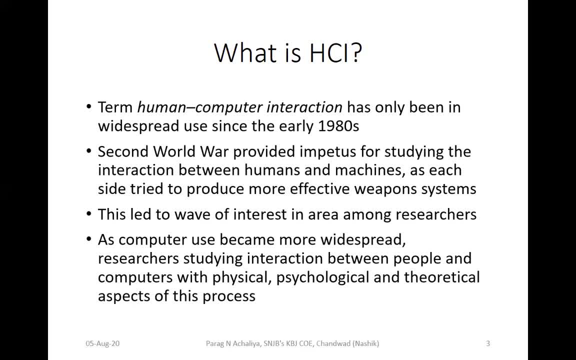 interaction. so the study of researcher start from physical, psychological and theoretical aspect. physical means how, how we are using our system. just say up message which makes physical aspect: yes, all the combinations are there. psychological means what? And in this way they've lost all their health Travel完. 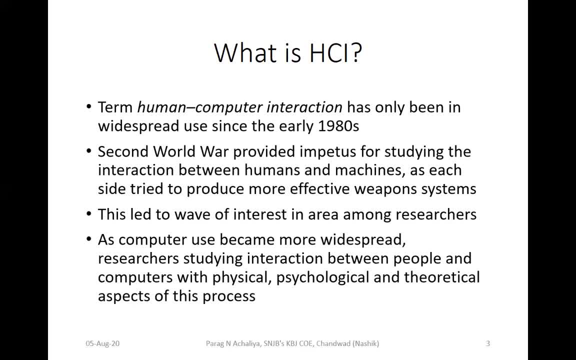 means what it will affect on your psychology. so this is what the psychological thing is, and theoretical aspect means what the theoretical aspect of hci is. so these are the thing where researcher started their study on physical aspect, psychological aspect and theoretical aspect of your what human computer. 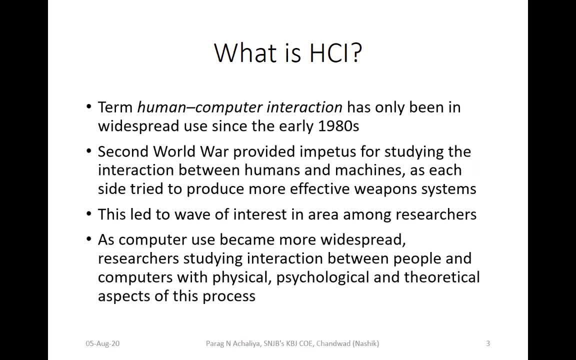 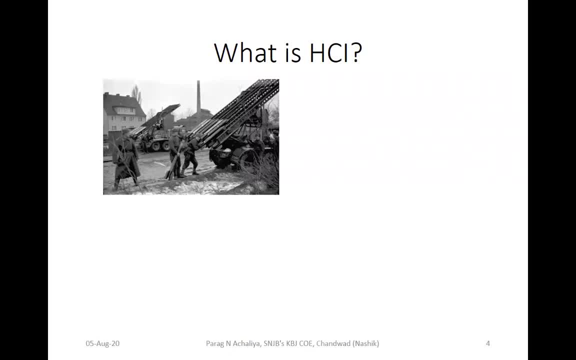 interaction or they start studying the interaction between people and the system or computer. you can see some of the pictures of world war now. see here in the first picture. in this picture you can see the people are using the machines. the size of the machine is much bigger than the people. 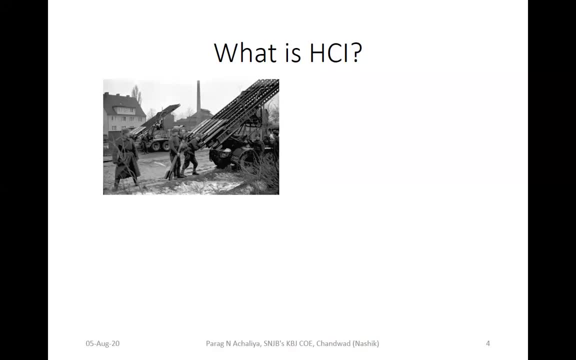 and that person is loading the rocket onto the on that rocket launcher. so now you have seen, in lockdown there was no machines. so what they did? they had Gada sword and shield and with their help they made the people create the shape of war and partially, there wereС homes between the songs. now here you will see. 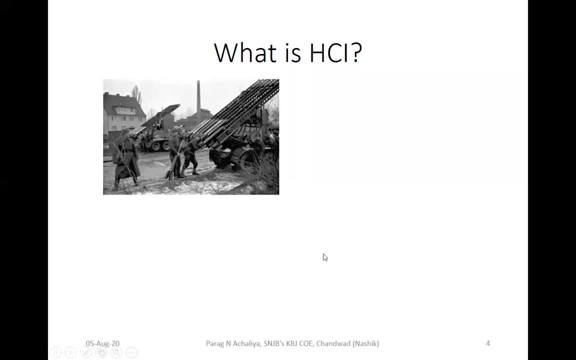 those machines are what its starting using the machine or the people were. use the machine for the purpose. like you can see this picture, what happens here? rocket launch. now, where 100 people were working, now only 3 people are working. so human efforts get reduced and the output will get increased. 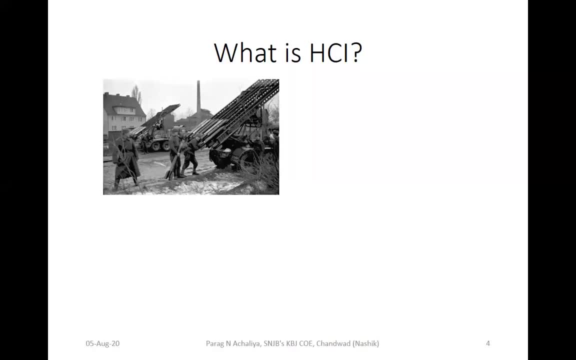 so after launching one rocket, 100 people die, and in traditional way, if there was war, then only one person could kill 2-3 people. so this is how the use of machine get increased in your day to day life and the human computer interaction starts from second world war. 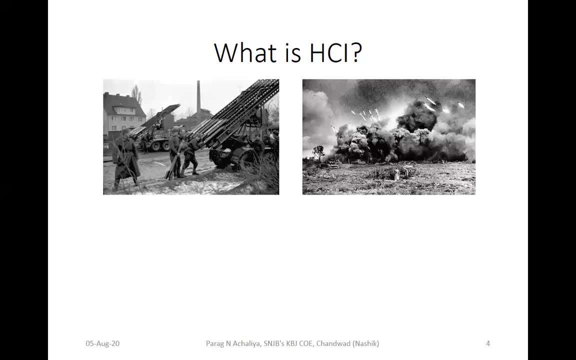 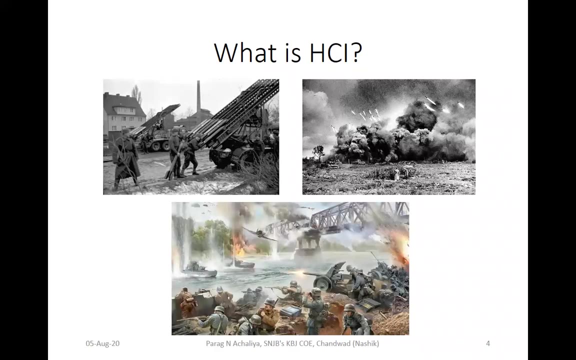 you can see this after rocket launch: what happens, what doesn't happen. now you don't need to discuss these things. you know this. you have seen in movies. what happens after rocket launch, what doesn't happen. this is how the damage occurs. how much damage happens. 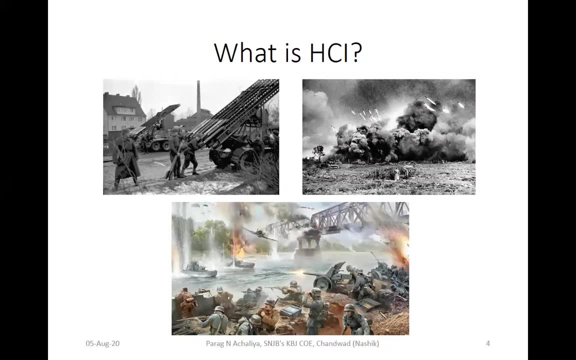 the whole bridge is broken or whatever happens. so this is what the use of machines and you can see. first the gun was a normal gun. now AK-47 has come. now the advanced version has also come in guns. in one click many bullets are triggered from there. 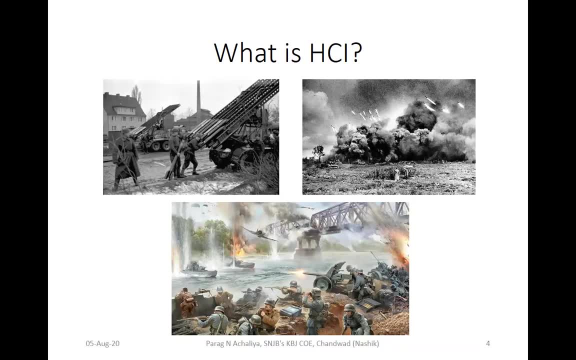 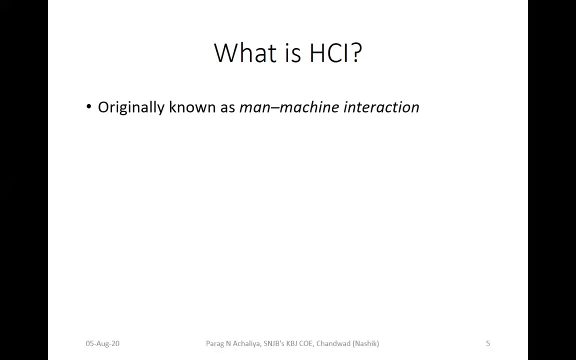 so this is what the use of machine and the use of machine get increased. you can see in your day to day life. you do the work of making work easy. for this you use systems. so originally it was human computer interaction. it was originally known as man-machine interaction. 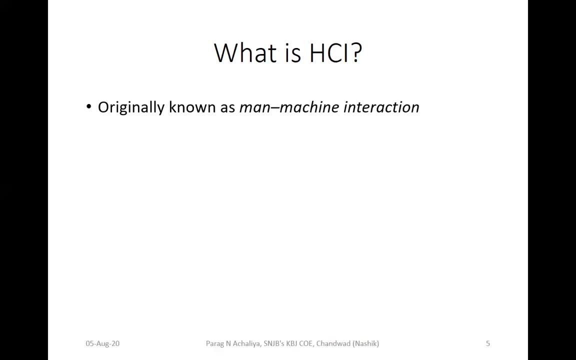 as I said in the beginning, it was human-machine interaction. as I said in the beginning, it was human-machine interaction. as I said in the beginning, it was human-machine interaction. it was the interaction betweenkus and system. it was the interaction between man and machine. 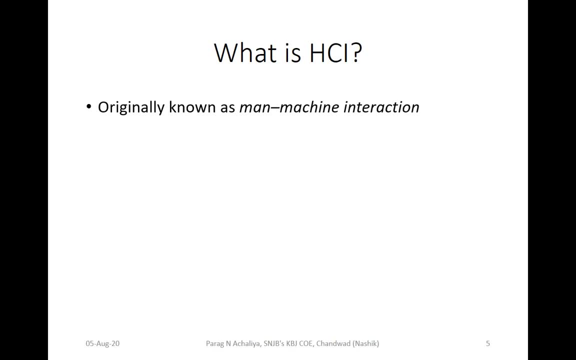 we can say that it was the interaction between man and machine, not only the machine. in broader terms, the machine can be your laptop, PC, your projector, 3.9x, your TV, IT engineering or computer engineering. we will specifically stick to machine will be your computer or it will be your laptop, or it will be your tablet. and now 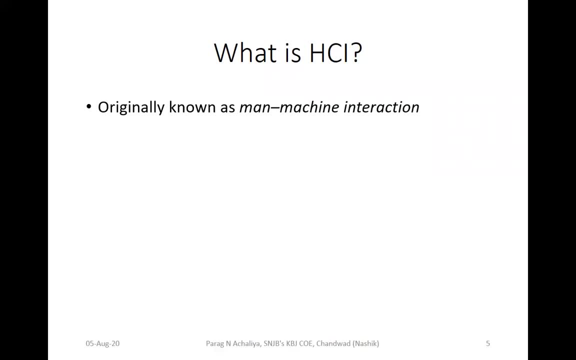 the machine can be your mobile device also. so originally or previously, man machine interaction was the name for your human computer interaction. later it became human computer interaction in recognition of particular interest in computers and composition of user population. this is a logo computers use: birthday guy. the man-machine interaction renamed with human computer. 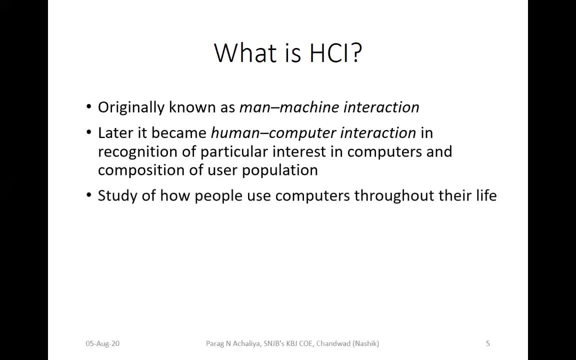 interaction. now we will call it as human mobile interaction. we may call it as human tablet interaction or human mobile interaction. so it is the study of how people use computers throughout their life, throughout life, how you are using your computers. it is the study of HCI, so HCI will be. 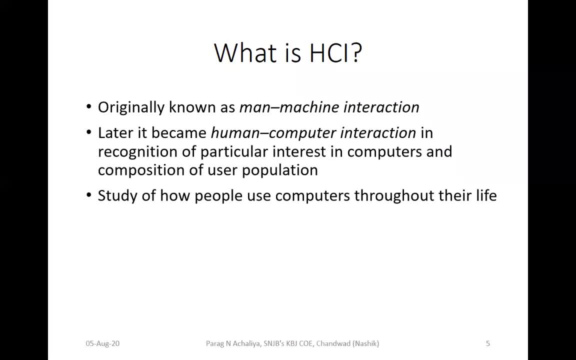 focusing on how people use computers throughout their life. it you see in whatsapp- do not like to type in to type, but the finder give the mic option. you speak on the whatsapp, you in text and message say conversation in text as required and you send it. basically, you are not able to do, guys, if you 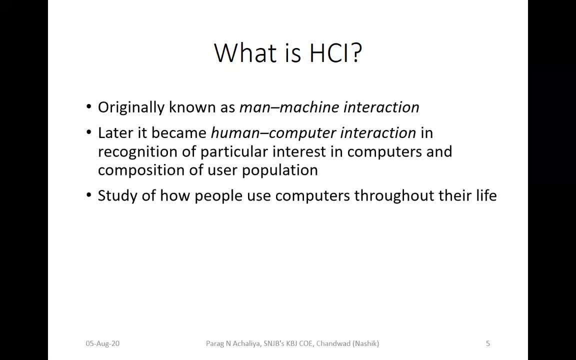 If someone likes typing, then it's okay. If someone doesn't like typing, like I am saying here, then whatever I say, if I convert it to speech, to text, then whatever I am saying here will be converted to text. So this is what we are using the machines. 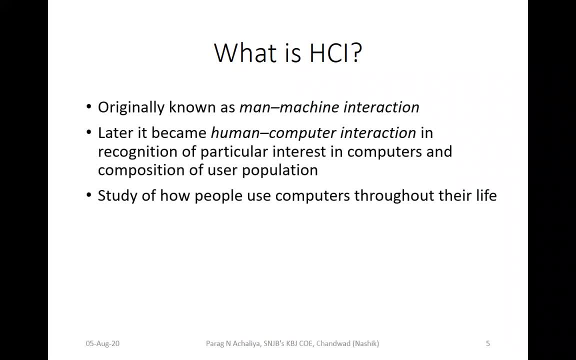 in our day-to-day life. So SCI mainly deals with how people use computers throughout their life. SCI draws on many disciplines in central concern of computer science and system design. SCI is present in many fields, Wherever you go. consider the example of building. 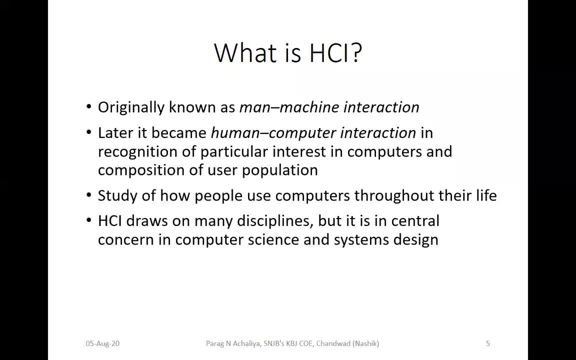 That is the example of civil engineering. Now, if there is a building, if you think about your room or imagine your classroom- It's been a long time since you saw your classroom, So imagine your classroom and the color of the wall in the classroom. 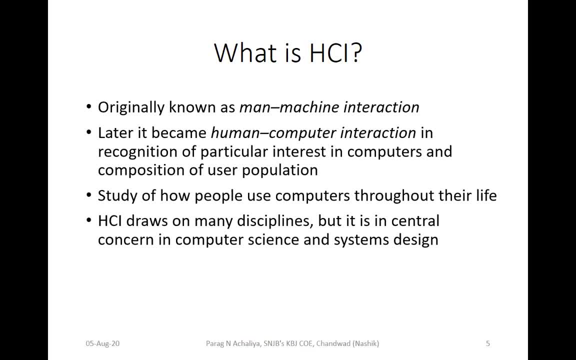 is of light color, Yellow color, off-white color or light orange color. It looks good. But instead of that color, just imagine that I am standing in front of you and you are attending the lecture and the wall behind me, the blackboard wall. 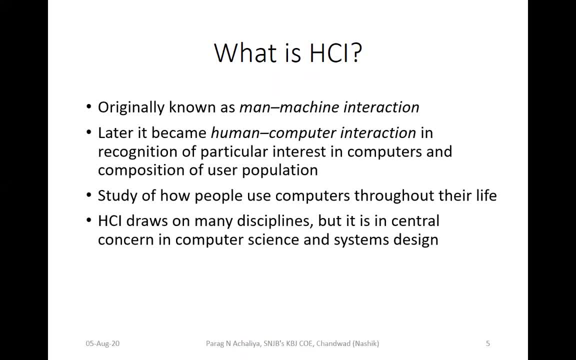 is in dark red color. So how it will look like, How will it look for your eyes? So there should be light color or dark color, The outer color of your building, the color of the building from the outside. how is it generally? 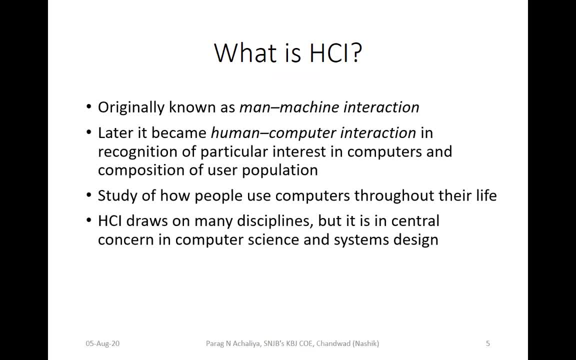 It is soft color, light color, Because it should look good for the eyes. So that is why HCI is mainly focusing on designing, system design, And that system design will be starting from your computer science Earlier, it was like this started building: 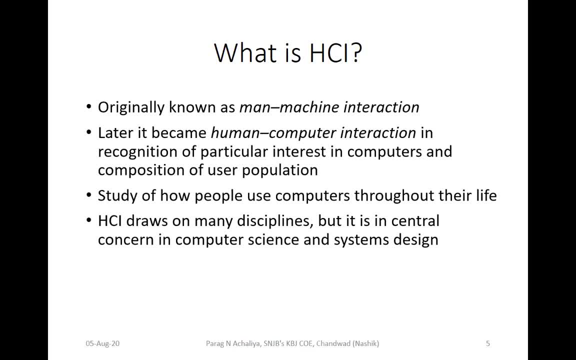 made a plan on paper plan approved. building started. Now civil engineers start using what Your AutoCAD or ProE software. With the help of those software, they are creating the 3D model of building That 3D model. 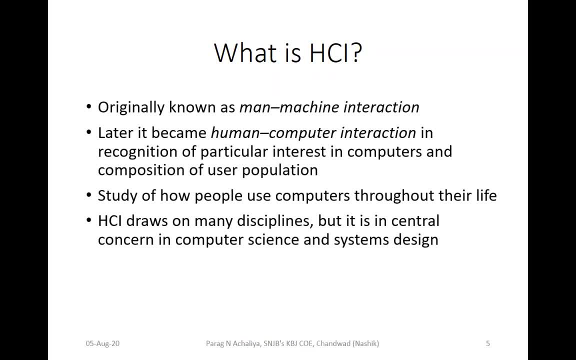 what do they do there? They give multiple colors. Which color combination will look good? Then they are finalizing that color. In the same way, if we consider the mechanical engineering, what happens in mechanical engineering? The mechanical engineers, whatever is the design of the car or vehicle. 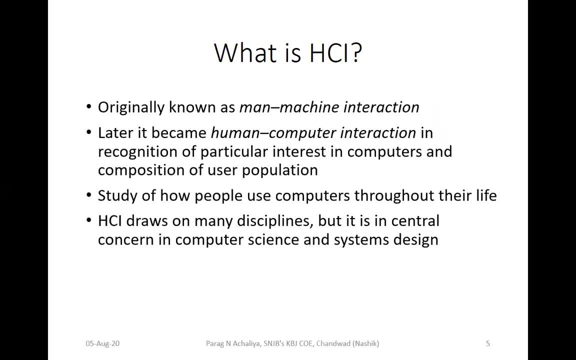 they used to draw that design on paper first. Now they start creating the design on computer system. Modify it as you want. Once it is good, then they start developing that system. So in every field computer comes into the picture. That's why this subject is very important. 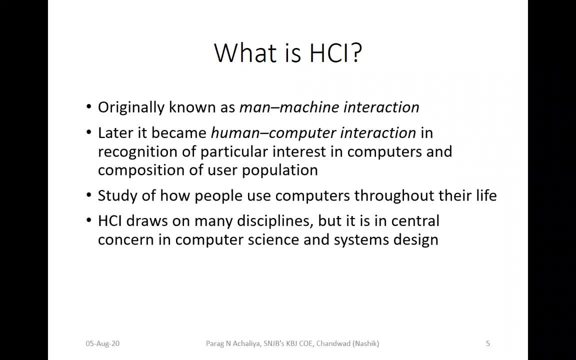 that how you are treating or how you are dealing with the computer system. So HCI comes in many disciplines and in every discipline the HCI will be at the central position, Basically in computer science and system design. Now see, here the word is system design. 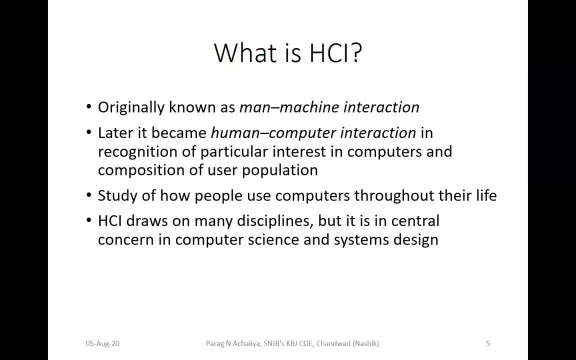 It is not the computer design, It is system design. So, as I said, the system can be anything: Your mobile fridge, TV, laptop, building, car, vehicle, anything. For all other disciplines it can be specialism. 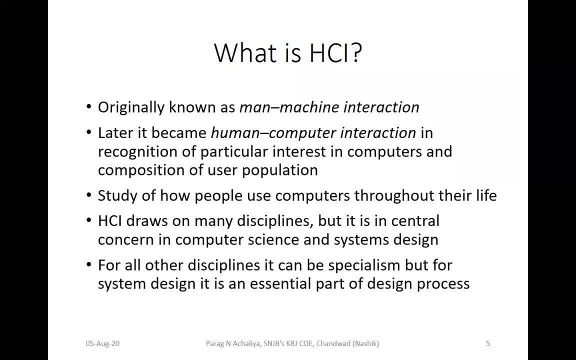 But for system design it is an essential part of design process. In the case of system design for other branches or other disciplines, it will be the specialization. What will be the specialization? There is a person in the company who will specifically work. 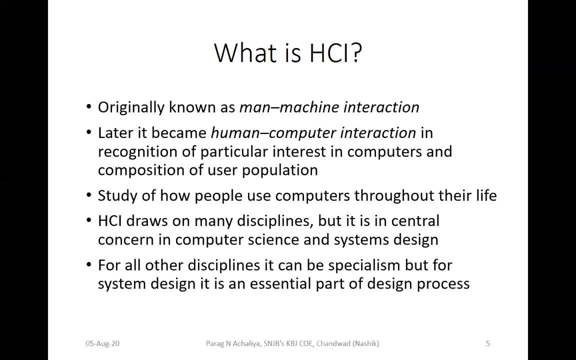 on the design, For example, if we think about the height of the car, the width, the diameter of the vehicle, the color of the car, the color of the seat, the color of the dashboard, Generally, the dashboard is 99.99% black. 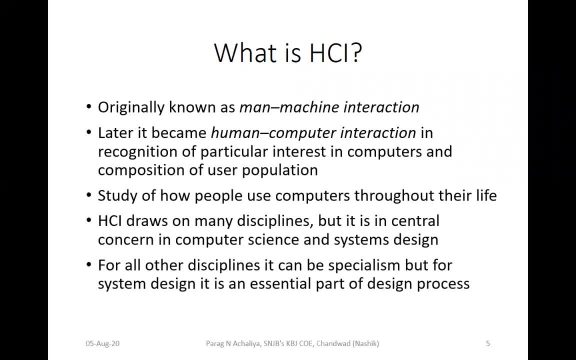 Why is it so? Have you ever thought about it? Why is it black? So these are the things. those are decided by the designer in that particular company. So for other companies it will be the specialization, HCI will be the specialization, But for we people, 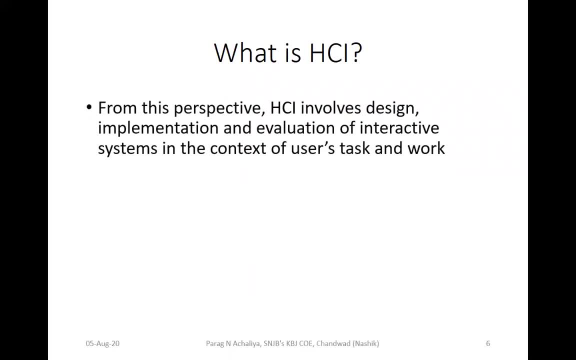 it is a part of our design process. For this perspective, HCI involves design, implementation and evaluation of interactive system in the context of user's task and work. So for we people, HCI involves three things. Number one: design, implementation. 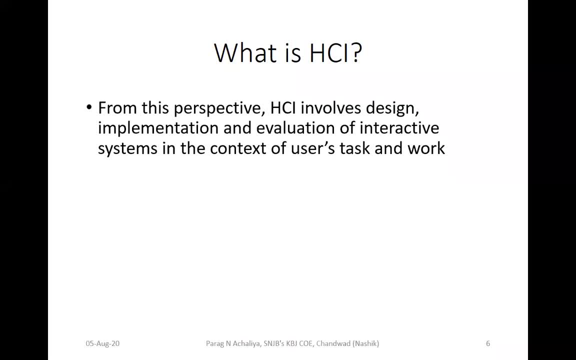 and evaluation. So what will come in the design? How should its design be? What should be in this design? What should be the color? What should be the font size? What are the different colors we can set for the text? Why is it so? 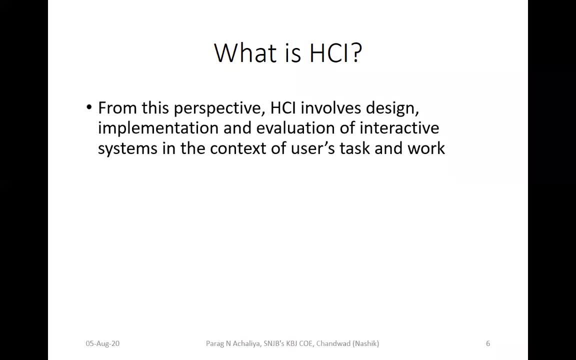 We are focusing on the design part. What happens in implementation, How we are implementing the system. After finalizing the design part, the implementation will start. And after completing the implementation part, the evaluation will start. Then, what happens in evaluation? Whatever system is developed? 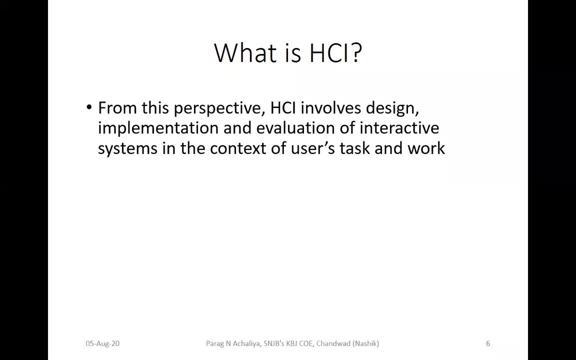 what do you do with that system? What do you do with various ways, Test it Whatever errors and problems are identified, and the design team and the implementation or development team start evaluating the system. Someone has some query, Sir. nothing is visible on the screen. 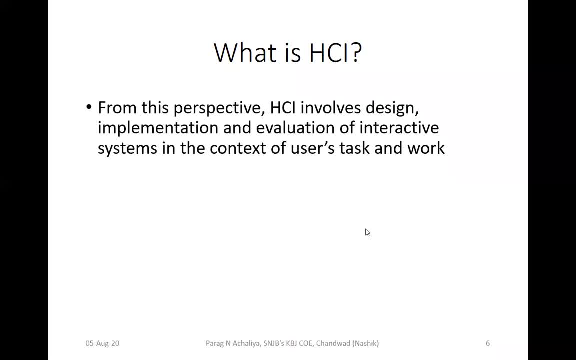 Whether the screen is visible, Yes or no. Please let me know whether the screen is visible. Yes, the screen is visible, Kavita, you can check from your hand. Yes, Pramod, tell me, Pramod, do you have any doubts? 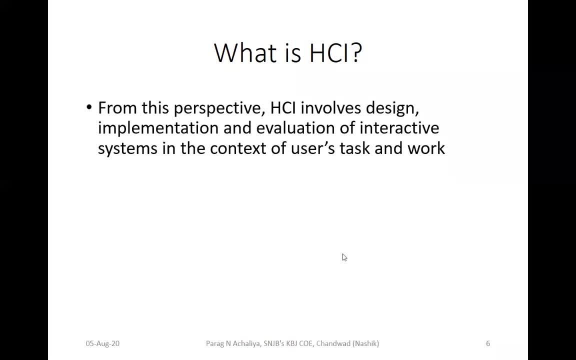 You have raised your hand, Okay. if you have any question or doubts, Please post your query or question into the chat box, because the recording is also going on. Please post in the chat box if you have any question. When we talk about HCI, we do not necessarily imagine single user with a desktop computer. 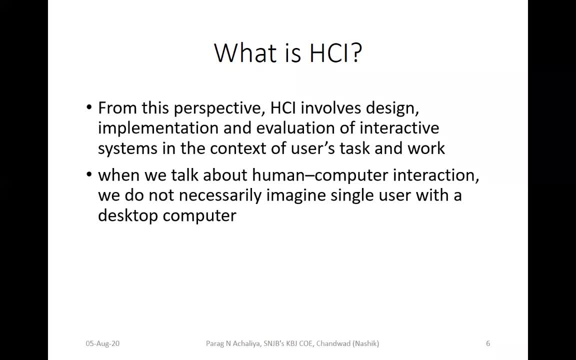 In case of HCI, always aisa nahi hoga ki there will be only one user and there will be that computer system or the desktop computer for that particular user. In case of HCI, it may happen just right now. we are communicating with each other. 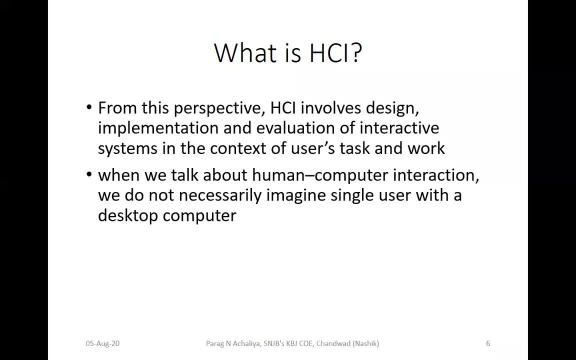 There are n number of users. We all are users and the system is your mobile, your laptop or my PC. So every time it may happen that right now in my laboratory, the HCI will be only I am the user and my system, But when we talk about this lecture, the HCI will be your. 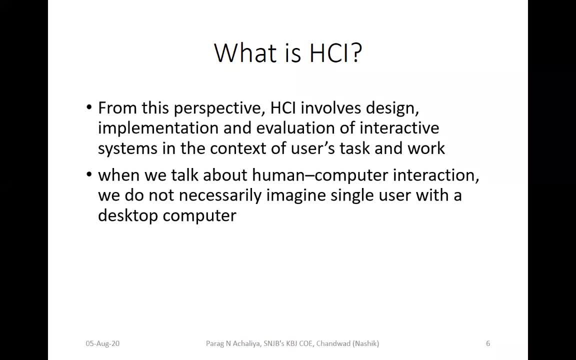 You all users. I am the user and the system we are using. So this comes into your what HCI- Human Computer Interaction- part. So who will be the user? A user can be an individual user like me or you. individual person or a user can be a group. 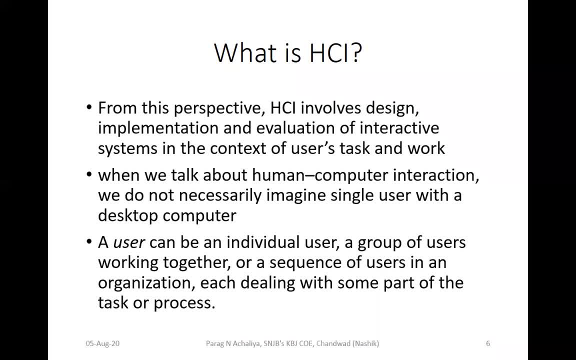 of users working together, just like a team Team mein. kya hota hai? Team mein 10 log, 5 log 2 log, 3 log Ek task ke upar work karta hai. So a user can be a group of users who are working together on a specific task, on a. 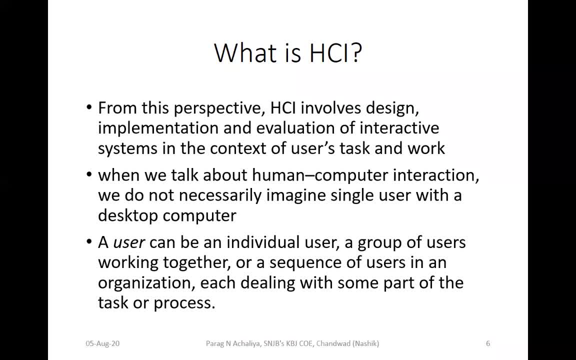 single task or a sequence of users in an organization. Sequence of users means what? For example, I am developing a software, There will be the team for designing. That designing team will handover that product to the development team. Development team will handover that product to the testing team. 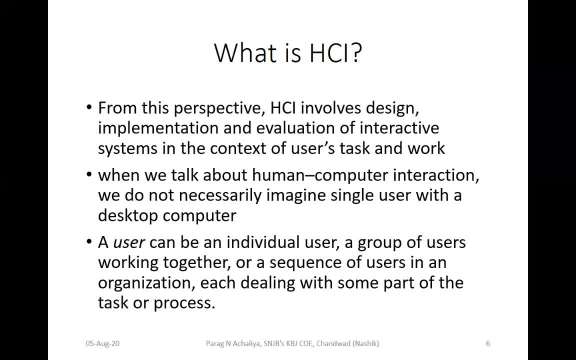 Jaise bhi development team ka task complete hota hai, that task will be assigned to the testing team. So this is the sequence. The sequence is following like design, then development, then testing and then deployment. So this is the sequence. 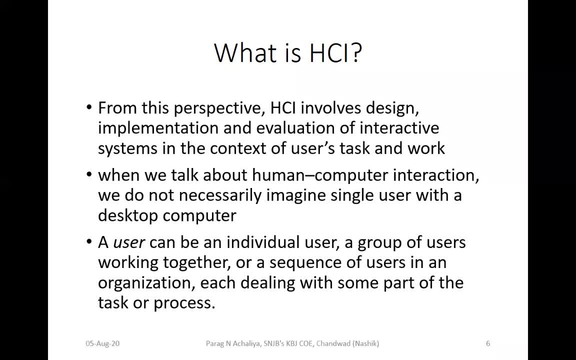 Jab tak previous user ka task complete nahi hota hai, next user will not work on that thing. That is the sequence of user in an organization In which each are dealing with some part of the task or process. So The single user, group of user or the sequence of user, they are going to deal with some part. 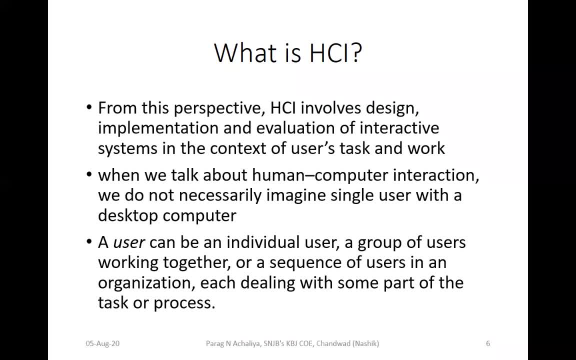 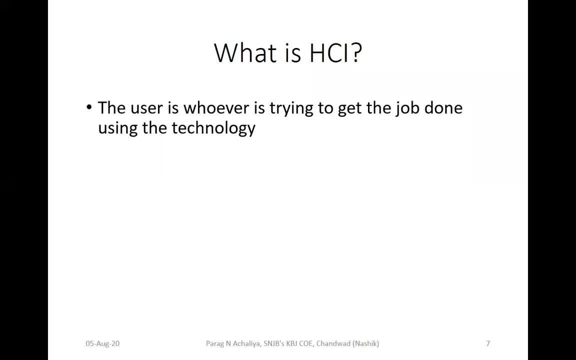 of the task or they are dealing with some task of the some part of the process. The user is whoever is trying to get the job done using the technology. Now, here the statement using the technology is very important. in case of HCI is concerned, The user is the person who want to complete a job, who want to complete his task. 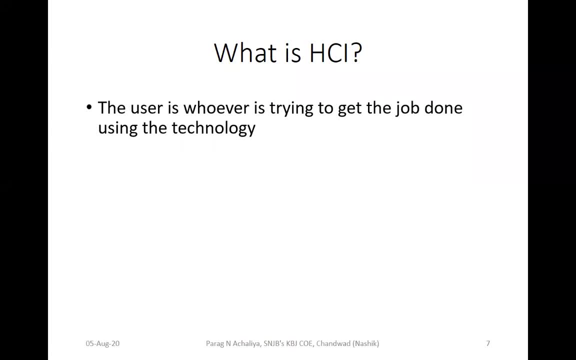 He may complete his task by traditionally also, or with the help of technology also. Now consider is semester. mein aap mini project karni wale ho. mini project, main aapko bula hai ki aapko apke project ke upar kya karna hai, report likhna hai. 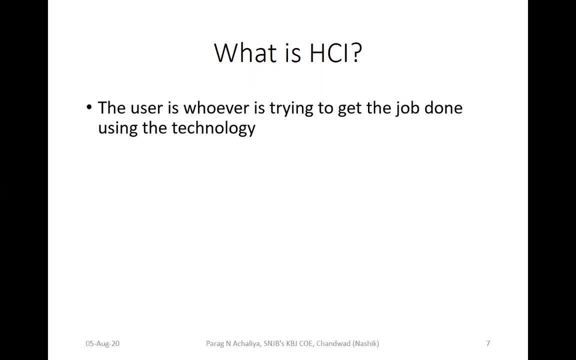 In that case, what you are going to do. there are two ways. Either you may start writing the report on your laptop or PC- This is using the technology- Or you may go with your computer and work on your laptop, Or you may start writing the report using the pen and paper. 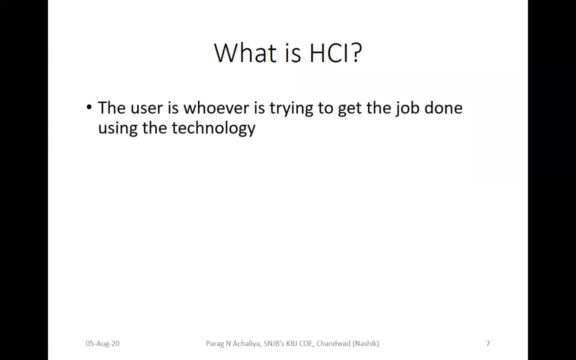 That means in traditional way. Now you will say that we are crazy to write with our hands and pen, As we have the computer system. So that is what the HCI is. You are starting the preparation of your report with the help of technology. 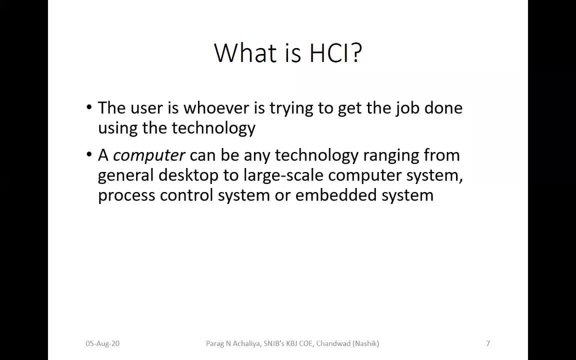 That is your HCI. A computer can be any technology, ranging from the general desktop to large scale computer system, Or it can be the process control system, or it can be your embedded system. Here computer doesn't mean only your PC. It can be the technology starting from our desktop system, mobile laptop or large scale computer system or process control system. 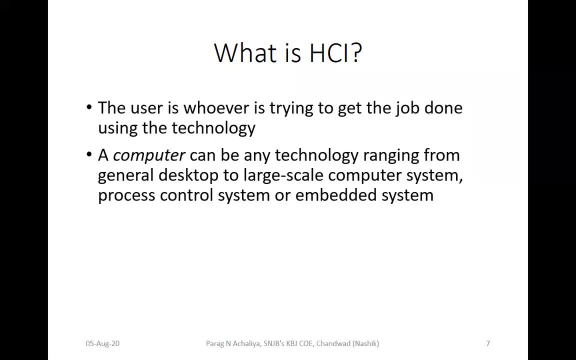 Process control system means, for example, your ERP. ERP is your process control system. You are giving some input And, with the help of ERP, You will pop some processes. You will get some output. ERP can be the example of your process control system or embedded system. 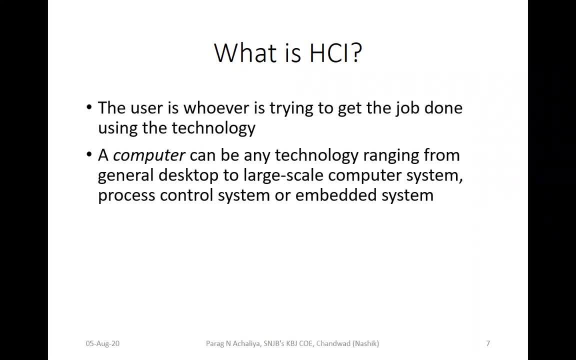 Embedded system is the combination of your hardware and software. Embedded system means your hardware and software, So we can call it as an embedded system. So the computer can be one of these things Which you can see on the screen. A system may include non-computerized. 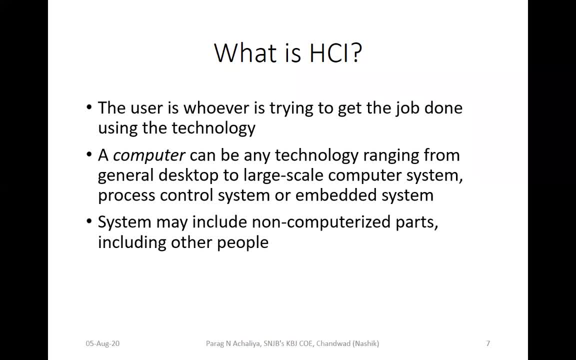 Parts, including other people. What can come in a system? A system may include non-computerized parts, Means non-computerized part. we can say anything which is not related with the computer, Just like our vehicle. Our vehicle will not always be connected with the computer. 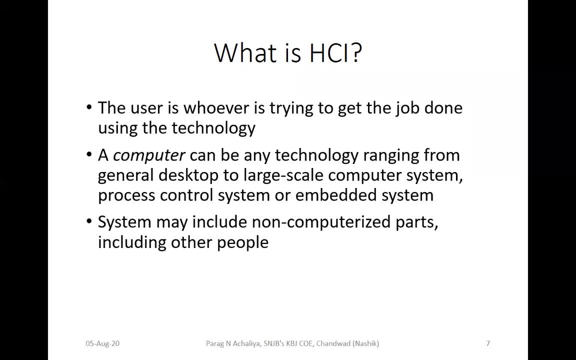 But it is a system. We can track the vehicle. Then it will become your computerized part, But at present We consider it as your two-wheeler. That will be your what System? or including other people? Other people may be in this online teaching.